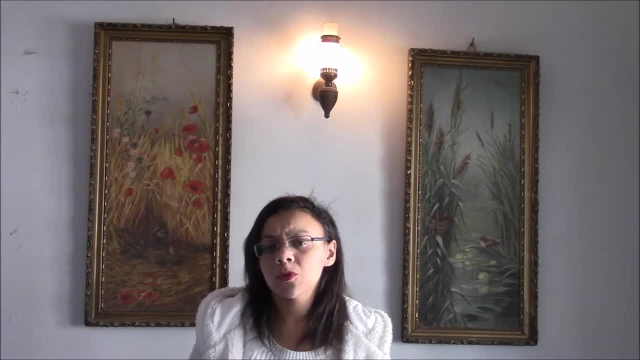 I prefer to film in the living room. My sister, 24-7, is in the living room so I can't get to film when she's there. So I try to film when she's not with me. and this is pretty hard because both of us work. I wasn't. 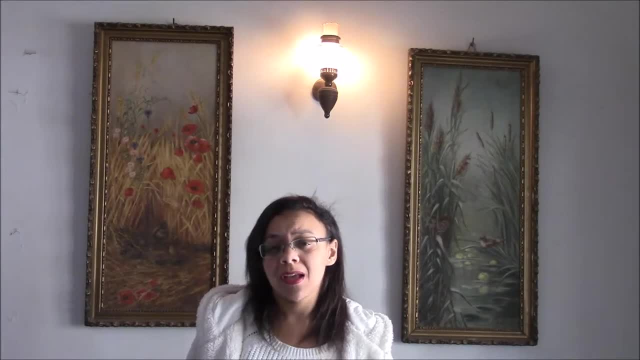 working for some time, but it was hard, and we will get to this in another video- to talk about how's life going and how can life get you done, and all of this stuff. So I'm not going to talk about this now, Let's get right into it. 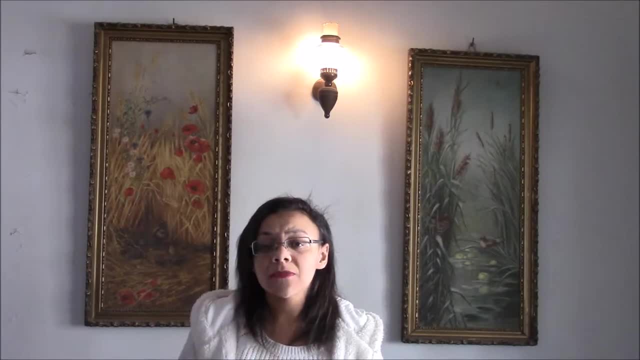 Let's get into the video. So first thing first. this video idea is inspired by Rafael Gomez. I'll link his channel in the description below because I love him so much. He's one of my favorite YouTubers, One of my favorites- I have so many favorites, actually, But yeah, So he made this video. 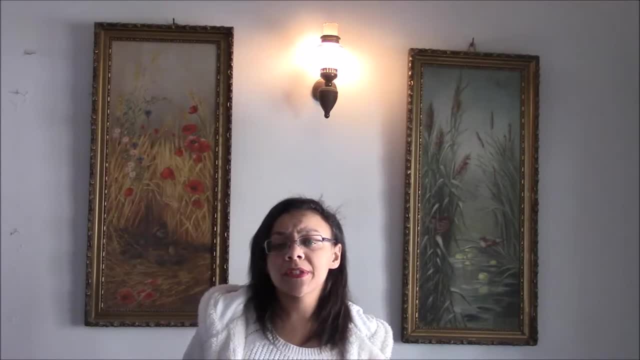 where he tried some foods used in hats, Hacks or things to fix everyday things. So I'll link this video down below, as I told you. But in this video he was wondering why these things work this way. because there's some they're weird. I can't say that this is weird And because I love science, maybe. 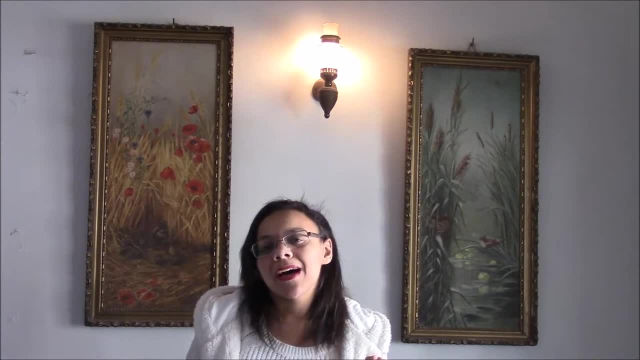 more than I should. I searched and I knew already some of them, So I thought I would stay up and talk with you about them. So the first thing that was in the video of Rafael. he got a video from another page that I don't know, But he linked it So I'll copy paste the link. I don't know the actual page. 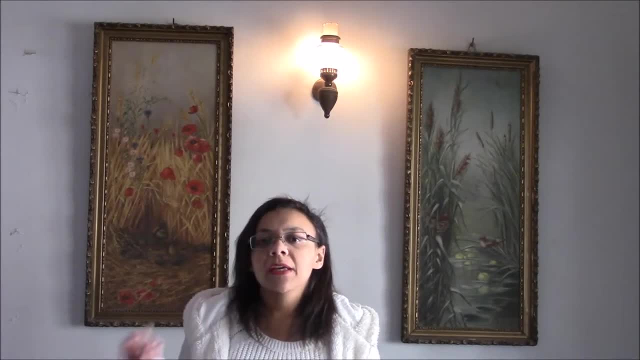 that posted or channel or whatever. So they're like the hacks that are used to fix everyday objects, But with facts, And they're funny and funny. So let's get started. So first thing that I'll say is how to clean it. 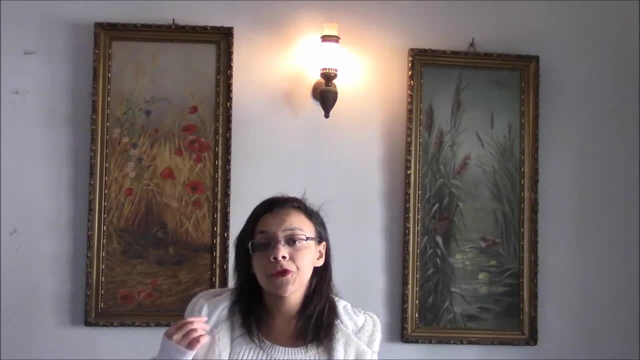 How to clean it first. HEY, SORRY FOR THE USER, I WOULD LIKE TO DANGER YOUR DEALWINDS. So to start with, first thing is how to clean paintings. dusty paintings with bagel- Strange, Absolutely strange. 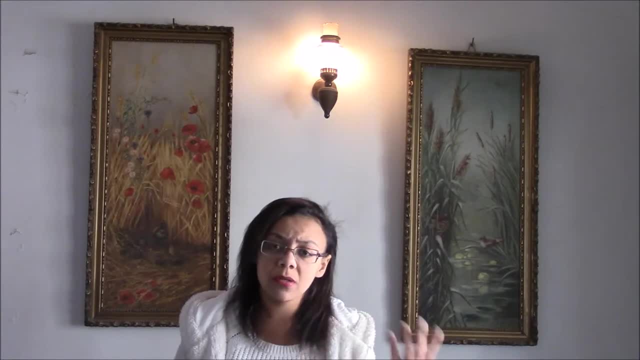 But when I was searching around painting and how to clean paintings and things like this, I found out- because I'm into art- How to clean, How to decorate, How to throw things away, How to clean, How to clean, How to clean. 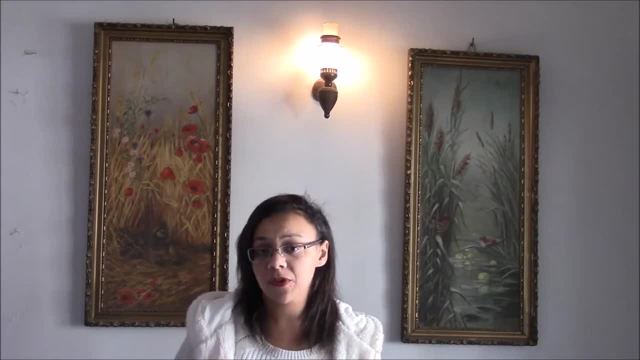 to. I like to draw and I have a drawing on canvas. I can show it to you guys sometimes. but I'm searching about this few months before and I found that a good way to clean paintings. put our potatoes- you can clean them with potatoes and like slices that raw potato and you just drop them through the. 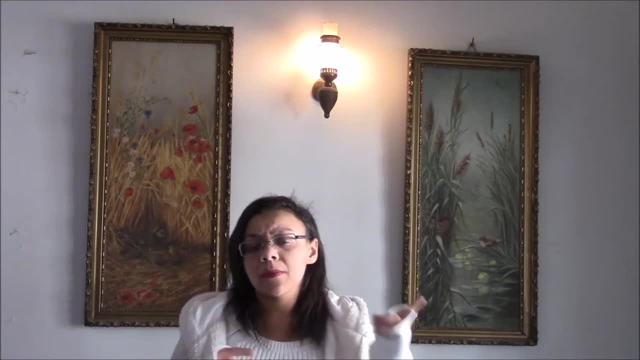 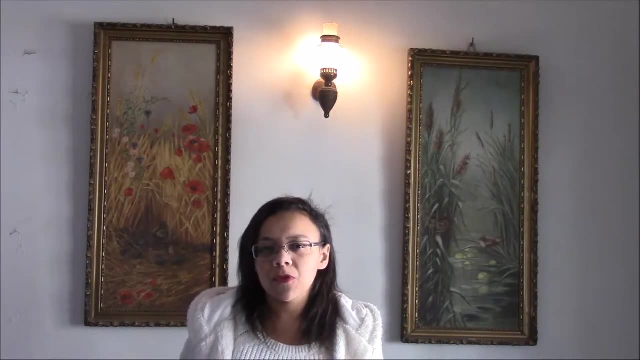 painting in this video. Rafael played another video of people cleaning with bagel, and I saw this video before and I kept wondering what's common between potatoes and bagel? actually, two things very similar. both of the- the bagel and the potatoes- both contains torch and this is because they have yeast. so this 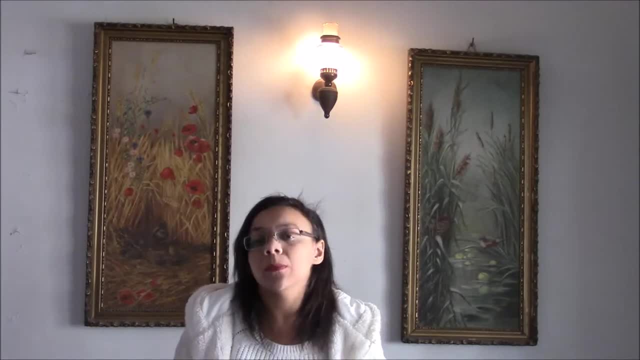 is why- this is the reason why I'm showing you this video- because I want to show you the main thing that helps and cleaning the paintings. so the thing that helps to clean in general is the torch found in the potatoes or the bagel. so why you? 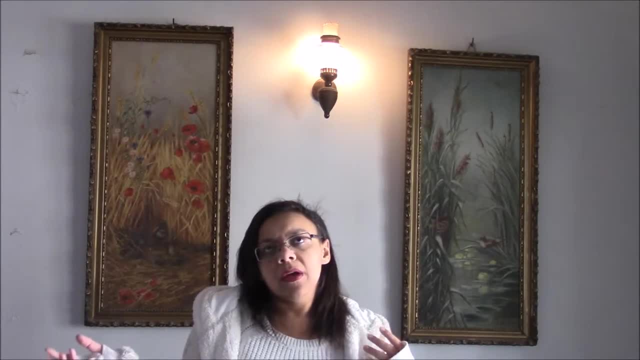 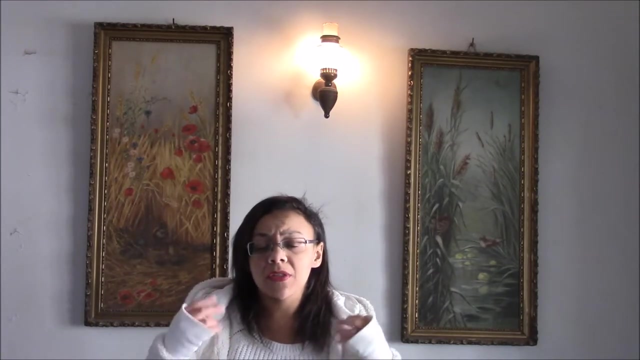 don't use a normal piece of bread. well, you can use a normal piece of bread, but the thing is a bagel. this is something like kitchen and cooking bologna kind of thing, not like any scientific thing. but when you make bagel bagels, the dough itself is harder, and this is this is because it doesn't contain much water. 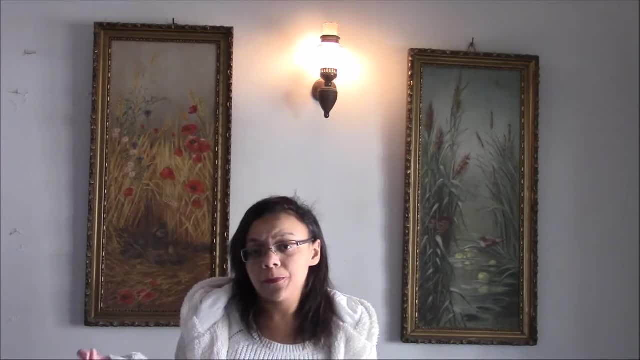 so this makes it clean better because it's more stiff so you can hold it better. you can get to hold it and drop through the paintings. second thing that we're going to talk about today is how to fix a broken plate with especially the China and the glass bits, things like this: how to fix them using milk. 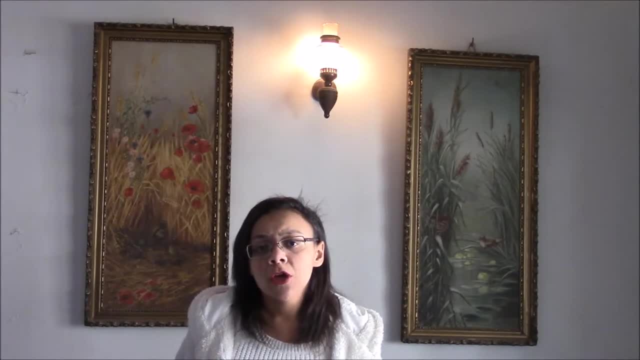 especially worm worm milk. so how this works. actually, I have a very interesting fact: ummers glue brand use milk, or two more precise, use a protein in milk. so let's make this more and more clear: milk consists of many proteins, and one of these is called casein. I apologize. 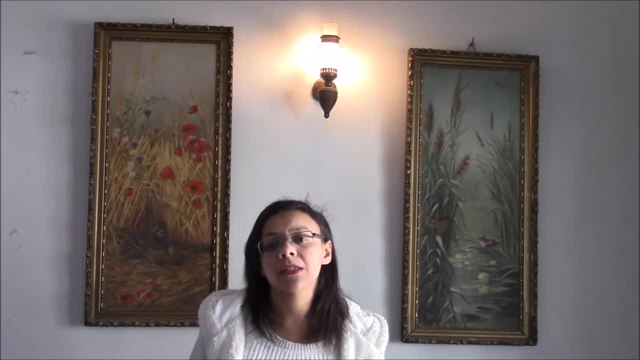 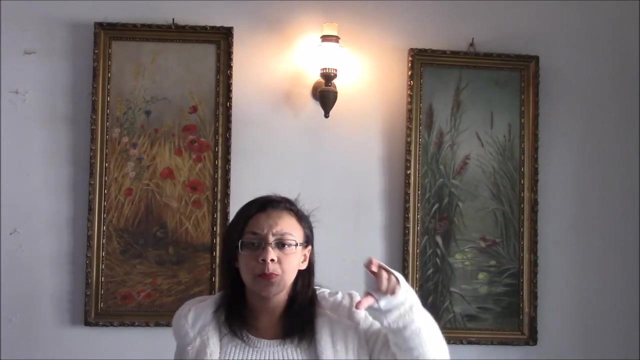 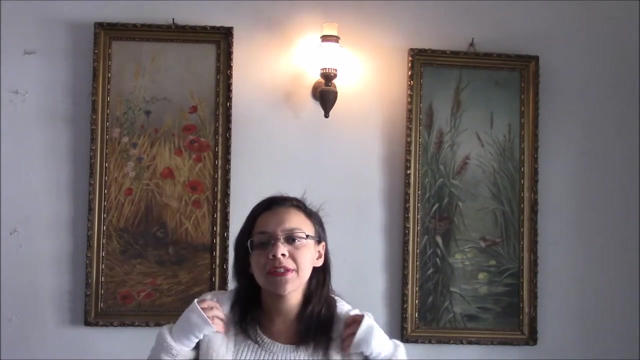 my pronunciation is not the best, but I think it's called casein, and this protein is known to glue things together. so when you need to worm the milk first, so you can't pour it from the bottom like this, you need to burn it first, like to give it a boil, then you can put it when it's warm. so why does this work? 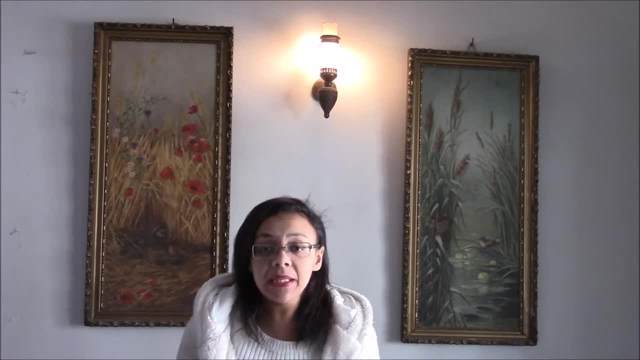 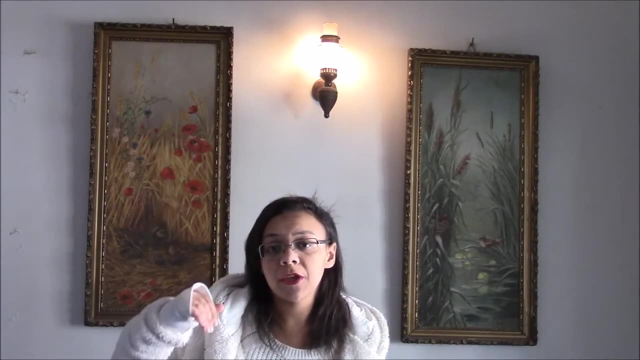 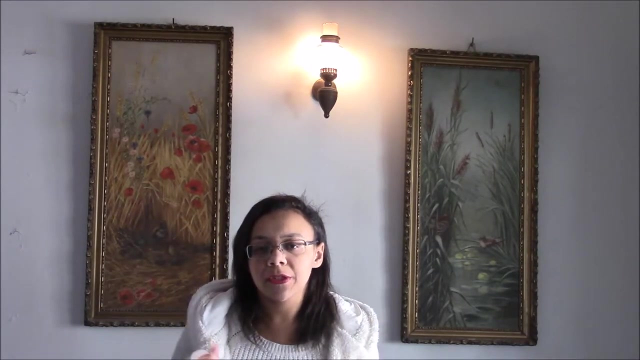 when you worm the milk, the proteins, the weaker proteins are the proteins. the weaker proteins are broken and they go to the up, to upwards. they go upwards in the container or the pot that you're using and because the heavier or the most resistant proteins go to the bottom. so what actually happens is casein is one of the heavy. 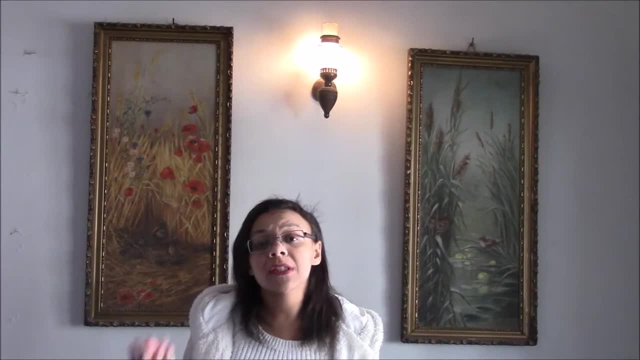 strong proteins and because it's strong, it goes downwards, it goes to the bottom. so imagine with me. you have a plate and casein is known for its use of known of gluing clicks, and it's used for this. so imagine with me. you put warm milk, so the 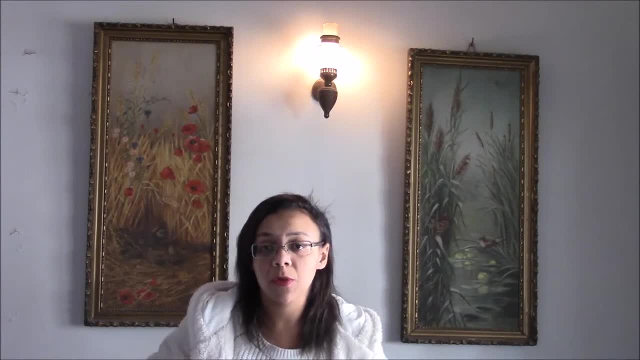 proteins, the heavy proteins, like casein is down at the bottom and you put this in with the broken plate that you already duct taped from the parts, like you put together with duct tape. so you only put them together with duct tape to ensure that it's in its place, that it will glue properly in its place when you pour the. 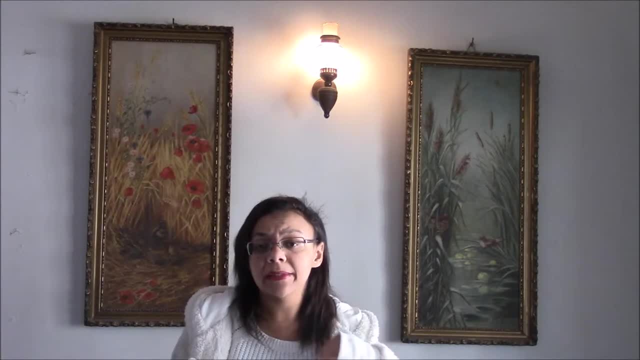 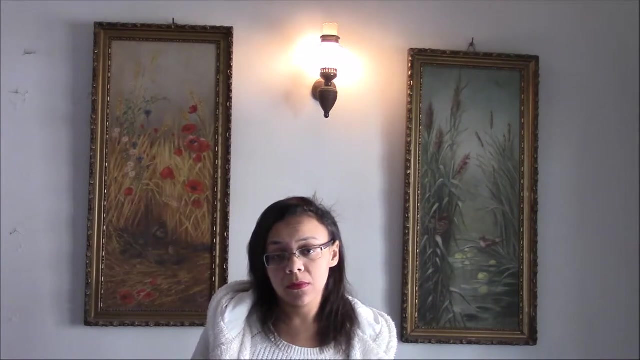 milk with the heavy protein and it's so it's down. the heavy proteins are down with casein, so this works as a glue. however, there's a different way that is used in making the glues. in general, Elmer's used to use casein, however, a 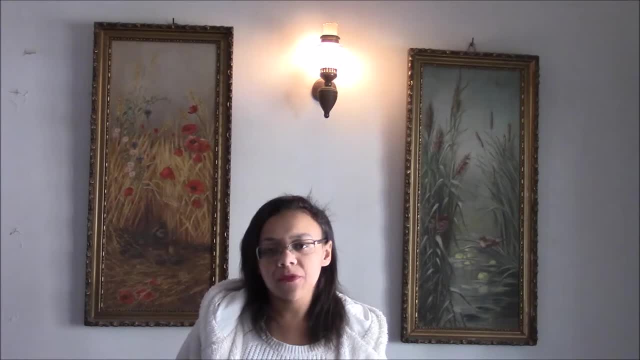 better way to use milk. you don't have to use duct tape for this one, because you can get warm milk and add vinegar. then you will realize that it's curdling, it's like buttermilk and, yeah, this will make it glue weird. yes, works, definitely works, which is good because 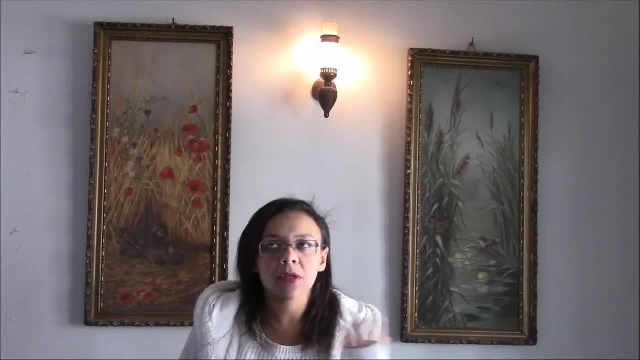 you can then use the plate again because it's not toxic, because it's made only of milk and vinegar, not not are toxic. they're both food. so you can safely use it again to serve food, and you can safely use it again to serve food, and you can safely use it again to serve food. and. 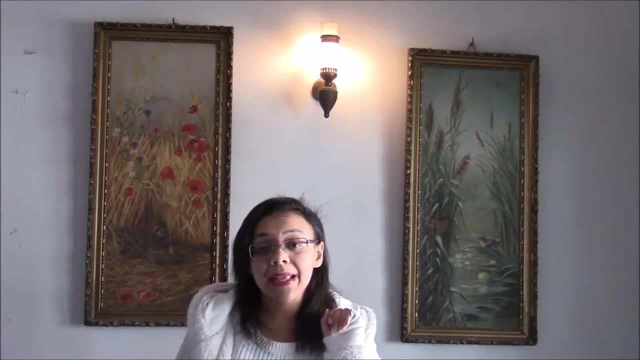 to eat in it. third thing that I'm going to talk about is how ketchup works with rust. this is pretty interesting because I knew before that vinegar is used to clear rust. when I saw the ketchup one, I totally thought about it like a ketchup. 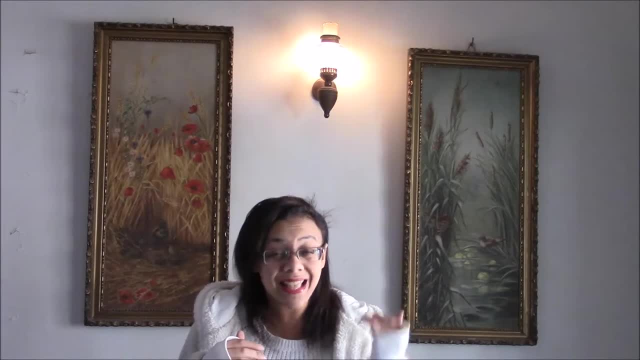 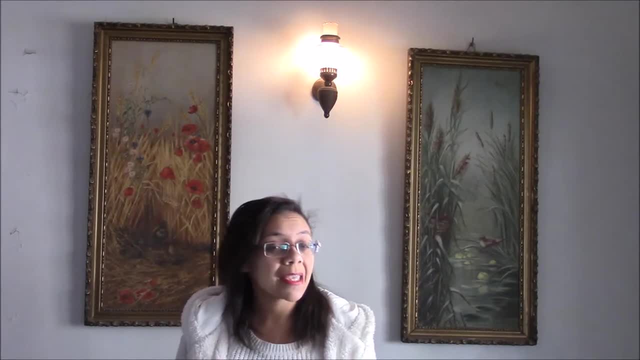 ketchup, so I wasn't that surprised. however, I kept asking: why are you seeing surprised? however, I kept asking: why are you seeing surprised? however, I kept asking: why are you seeing ketchup to clean the utensils, ketchup to clean the utensils, ketchup to clean the utensils, and not just vinegar? the answer is: vinegar or. 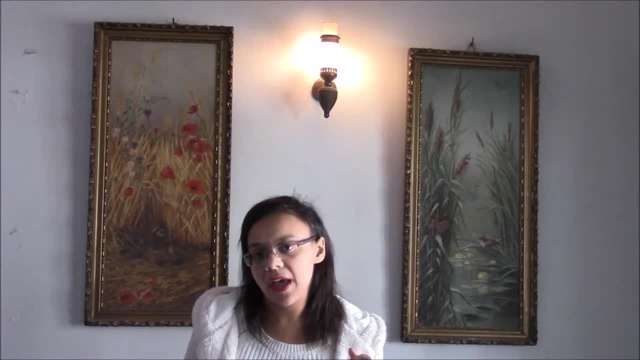 and not just vinegar. the answer is vinegar. or, and not just vinegar. the answer is vinegar or acidic acid kills the rust, and I have. acidic acid kills the rust, and I have. acidic acid kills the rust and I have a. it's scientifically written. I'll show it to. 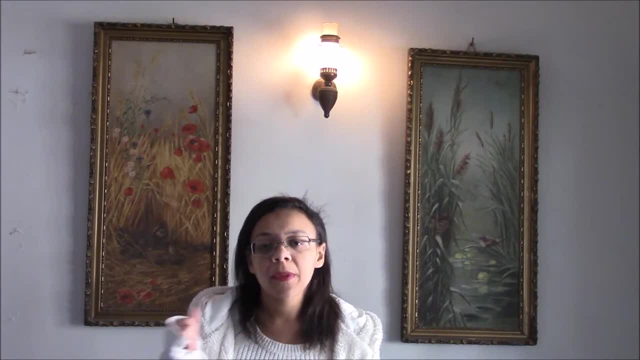 a. it's scientifically written. I'll show it to a. it's scientifically written. I'll show it to you first. why ketchup? why not vinegar? you first. why ketchup, why not vinegar? you first. why ketchup? why not vinegar? because a the ketchup contains all. 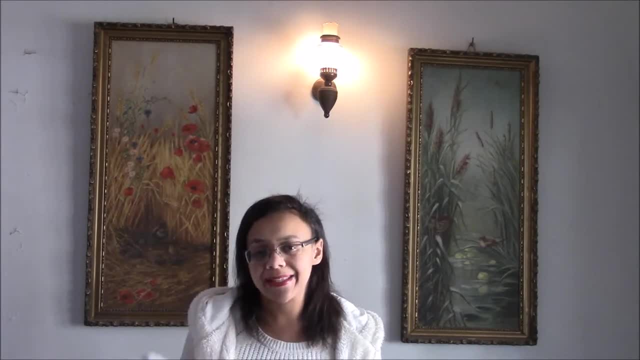 because a the ketchup contains all tomatoes. tomatoes are acidic, so it helps with the whole process to make the essence work with the rest and the main thing is the viscosity of the ketchup. because vinegar is so liquidy you need to soak the utensil or the metal thing. 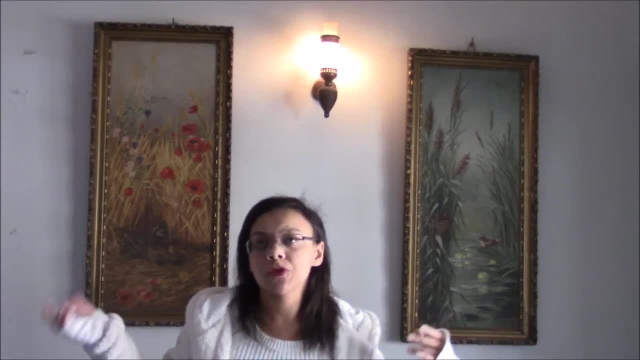 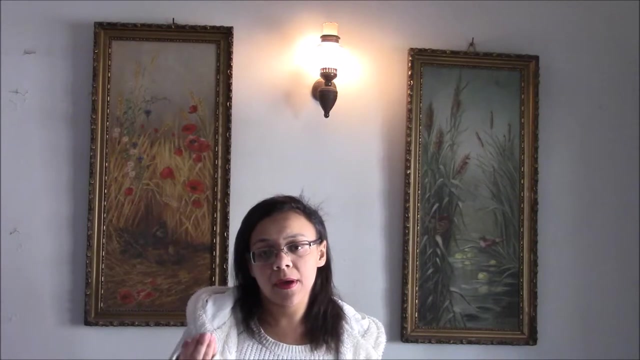 in it. so if you have a huge metal pot that you want to get this rust away from, you need to soak it in lots and lots of ketchup- I'm sorry of vinegar. however, if you have ketchup, you can get a whole bunch of ketchup or some ketchup. 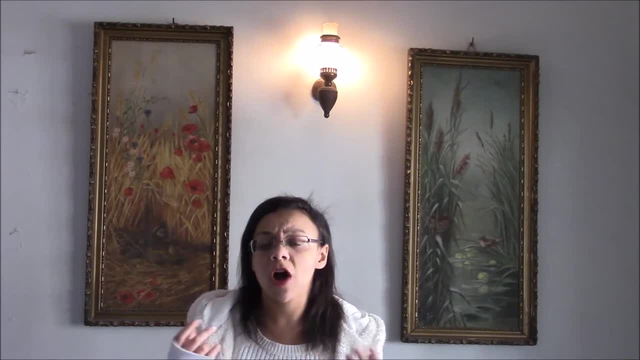 and because it's because of its high viscosity, so you can rub it and not soak it, so it will be more efficient. we're not done with this yet, because I need to show you something chemical. it's chemistry and I love chemistry, so let me get something for. 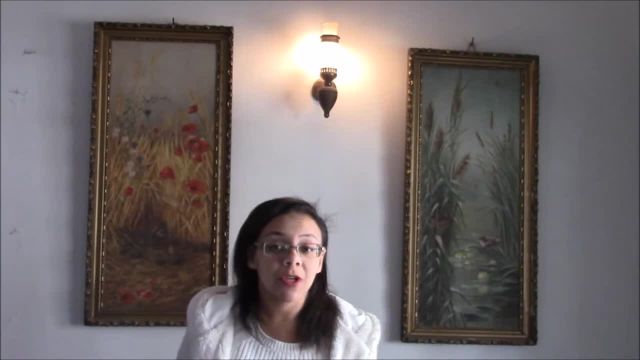 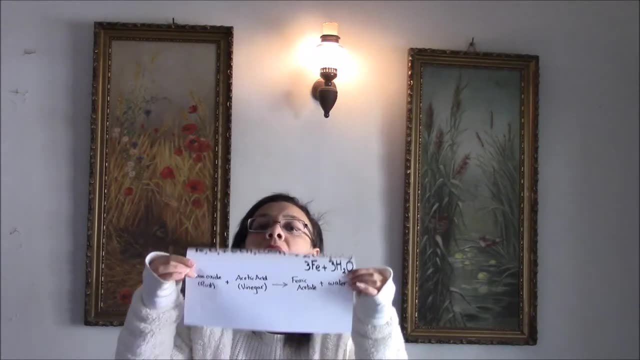 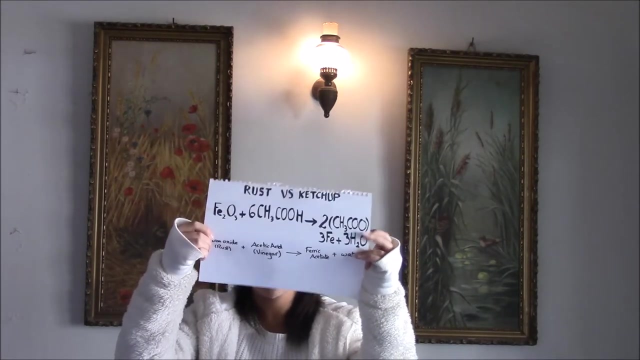 you, and at this point I don't care for you to see my face. I want you to see this paper instead, and I hope you can see it focused and well, can you see it? I hope so. so this is Fe 2 O 3. this is iron oxide, and 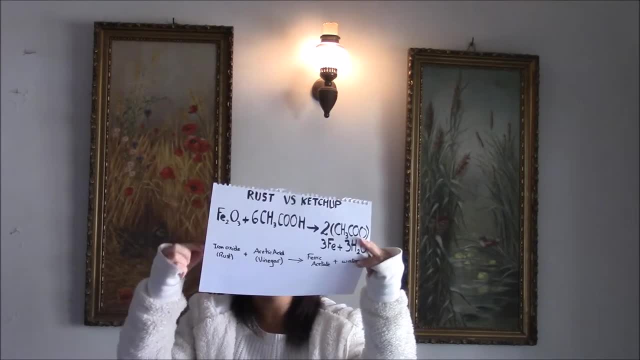 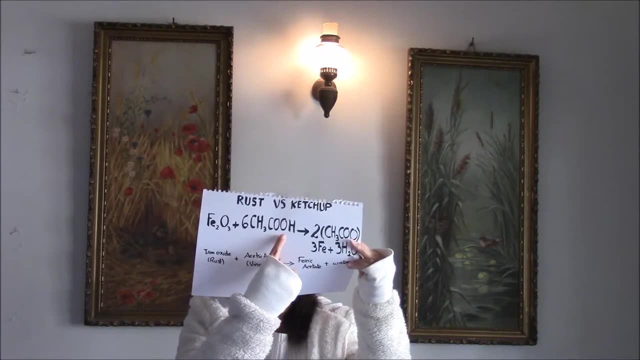 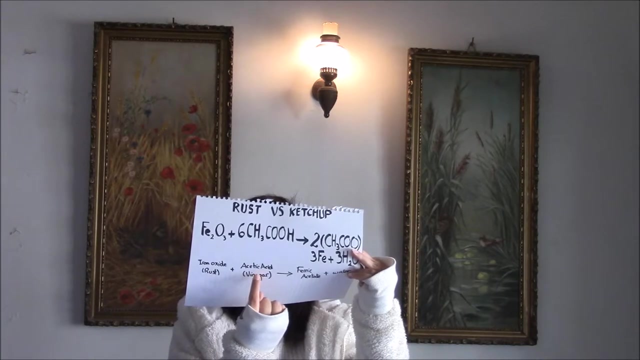 this is, this is this is the formula or the chemical name for rusts. then c, h, three c, o, o, h. i'm spelling it because i'm not sure if it's clear. here is acetic acid, which is vinegar, which we said before. that it's what. 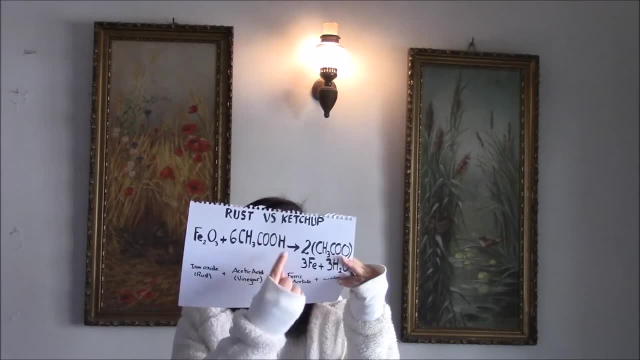 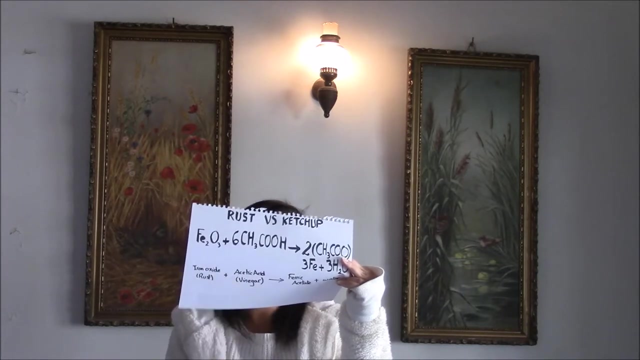 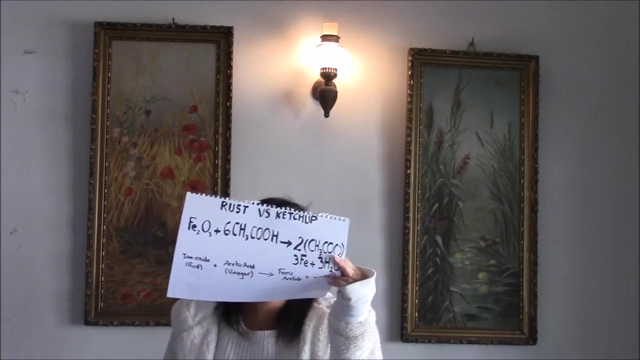 works? what makes the ketchup works? so, um, basically, there's a reaction that happens between iron oxide, which is the rust, and the acidic acid, which is the vinegar. vinegar, which is the acid, works on the iron oxide and it gives ferric acetate and water, so the ferric acetate just dissolves. 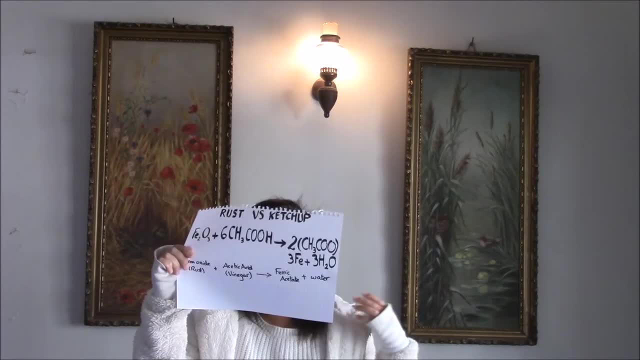 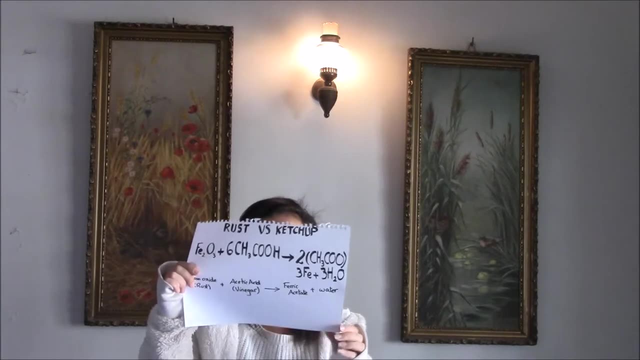 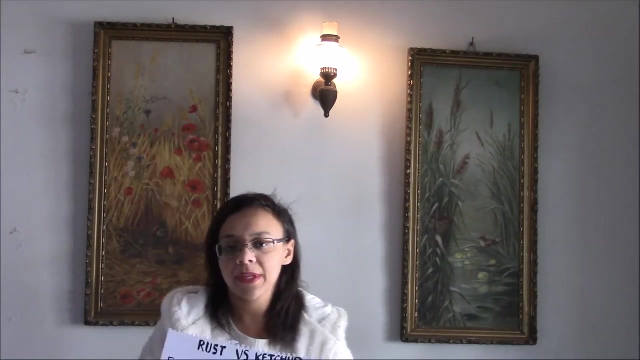 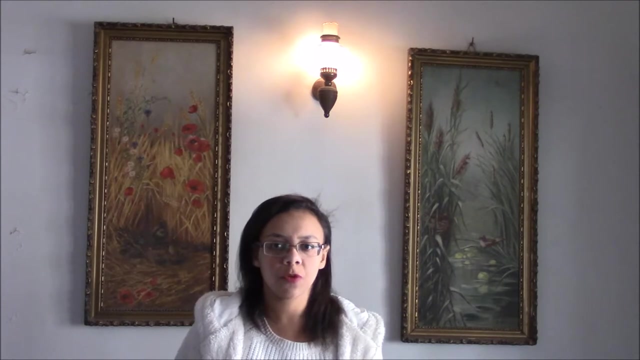 in the um, vinegar, or, in this case, ketchup, because it's more, it has more viscosity, and then water, which is perfectly fine. however, they're saying like: as this is how it looks like, i hope it's focused, okay. so, um, there's a like, an advice: if you use this at home, the ketchup one or the vinegar. 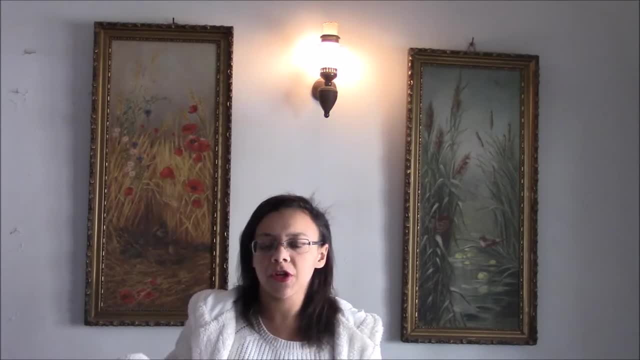 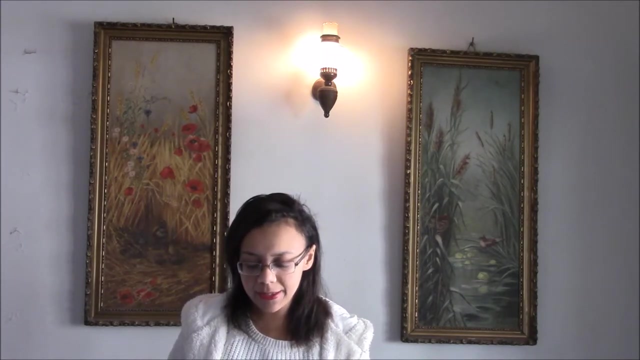 one. if it's something small, you can soak it in vinegar, it's fine. however, it's advised to use on the pot or the thing that you used, after you use the vinegar just to neutralize the effect of the acid. so for our fourth thing today, we have a really interesting thing. this is another scientific 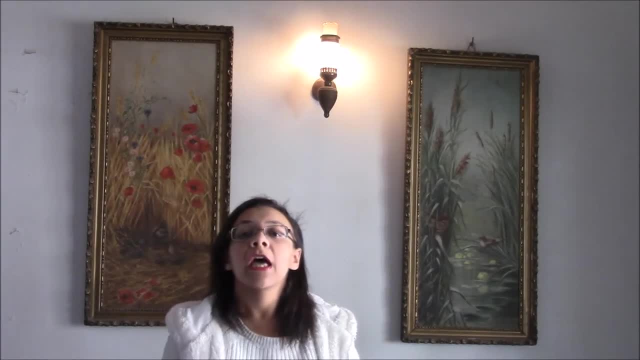 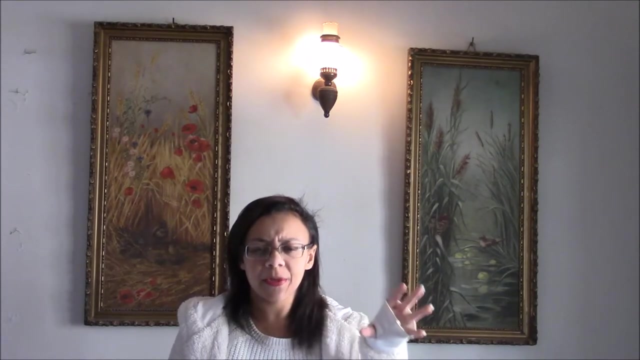 thing, which is cleaning a shower head with vinegar. so you get the shower head when it has these white particles, annoying white particles that um precipitate on the shower head and you want to clean it. so how do you do this? you get the the head, the shower head. 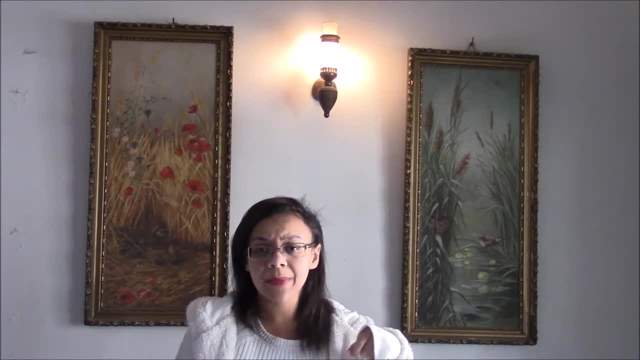 and you wrap it in a plastic bag or anything really with vinegar in it and wait for a few hours. then you can, after waiting for a few hours, it's soaked, it's nice and dry and it's okay to remove it and open the water, rinse it. so why does this? what's the? 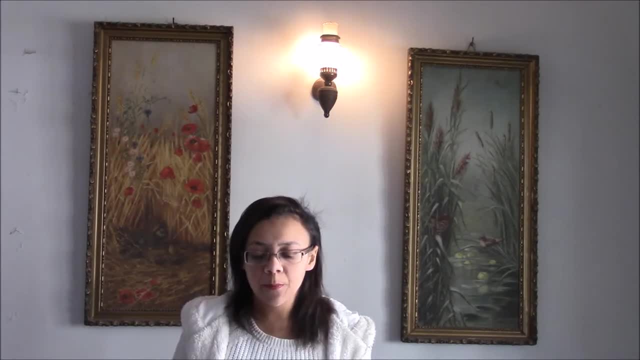 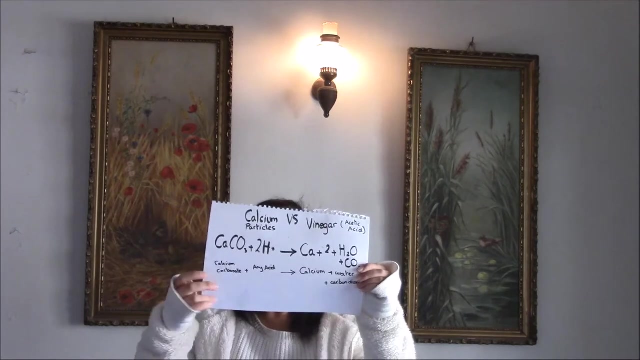 science behind it. the thing is, these white particles are calcium particles. here is the formula. i'll talk about it later. calcium particles are basically a form of calcium carbonate. calcium carbonate and calcium carbonate reacts with the vinegar, giving calcium plus water plus carbon dioxide. so this is how it works. calcium carbonate, which is like a the lime thing. i forgot the name, it's. 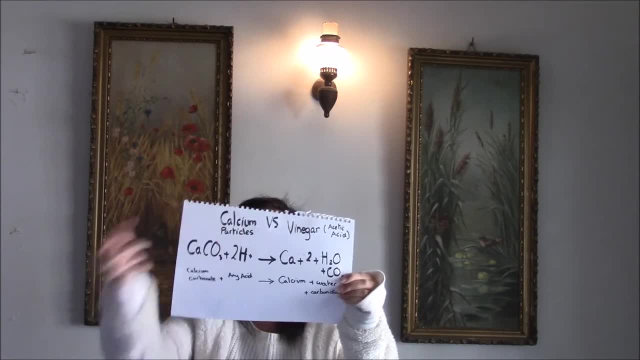 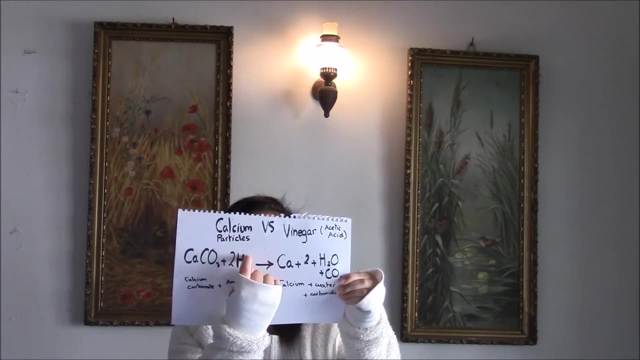 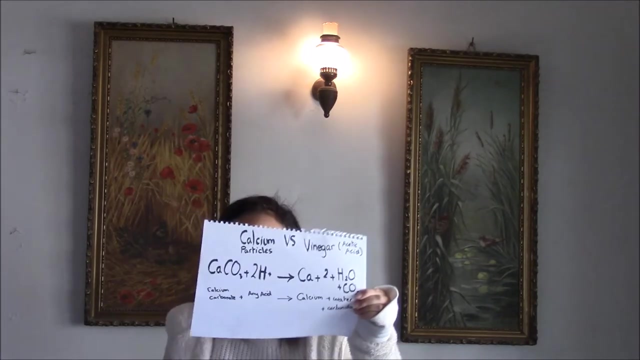 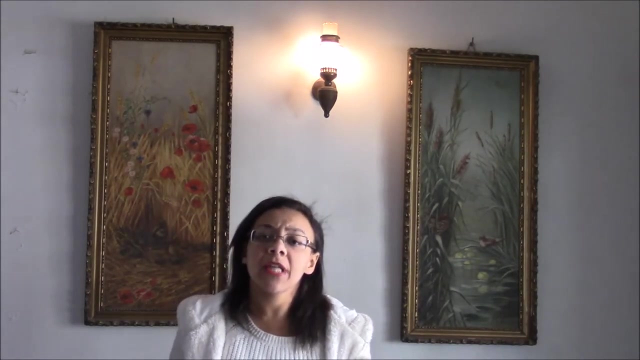 called lime particles or calcium particles, and basically why it's 2h and the plus is above here. it's not like i'm not adding something. it's above here. so h plus is um. it's an indication for any acid whatsoever. it doesn't have to be vinegar, it it has to be something. 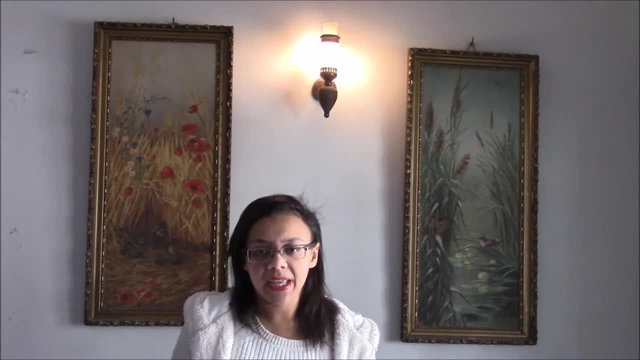 that can be soluble in water or water based acid. why you say because we need them to when it's it reacts with the calcium carbonate. we needed to produce the water in the carbon dioxide in order to get rid of the calcium carbonate. so because the hydrogen of the water will go from this one, from. 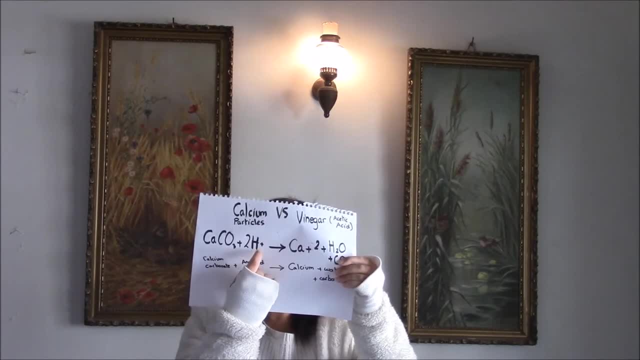 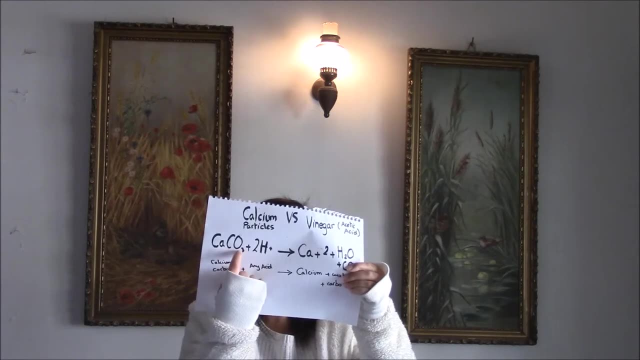 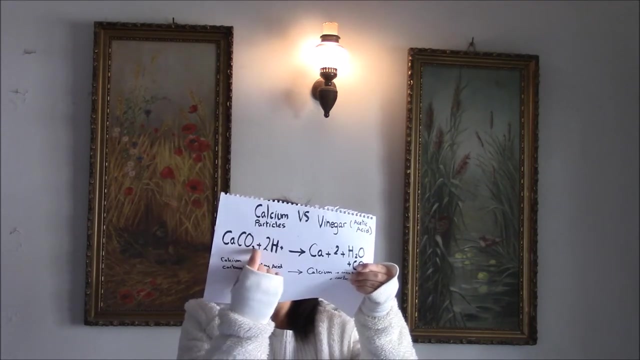 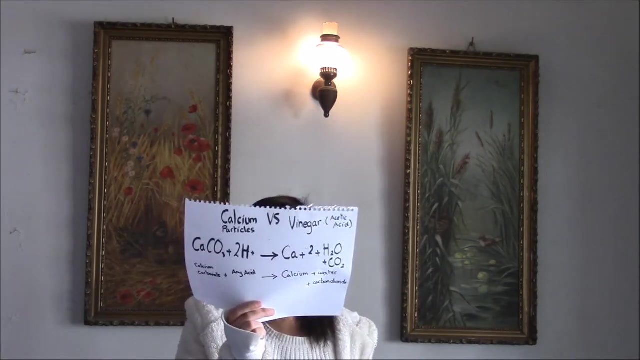 the any acid from the hydrogen molecule, of any acid, and will combine with one of the oxygens in the calcium carbonate and the other carbon here will combine with the other two here, giving carbon dioxide, and then the calcium will be all alone. okay, so after you add any kind of acid whatsoever, 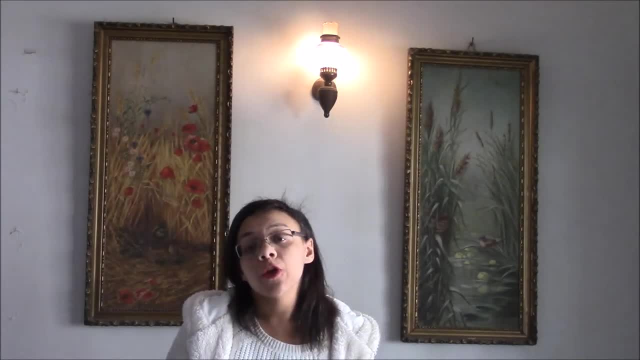 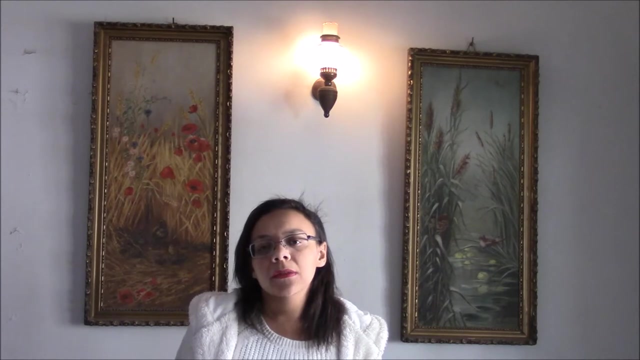 that can be in water. then you will get calcium particles plus water, normal water and carbon dioxide. carbon dioxide is a gas that will fly away and evaporate or go away and, um, yeah, water is normal, normal, totally normal to have it. and then calcium particles are just particles that are that. 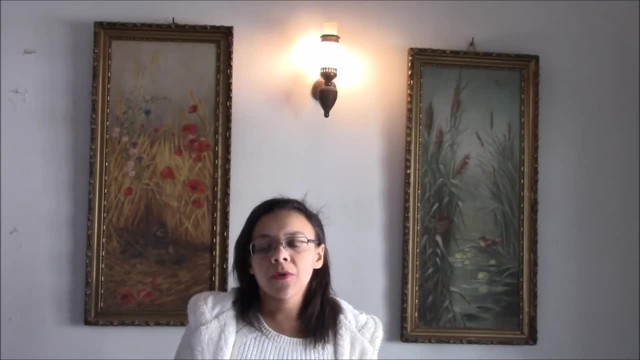 will remain in the water. so this is how it's cleaned. after you finish- uh, soaking it in the vinegar- you will find the bag it's. it doesn't smell like vinegar anymore- the bag itself- but the house will be smelling of lots of vinegar because you have soaked it for a few hours there and um, personally, i hate vinegar. 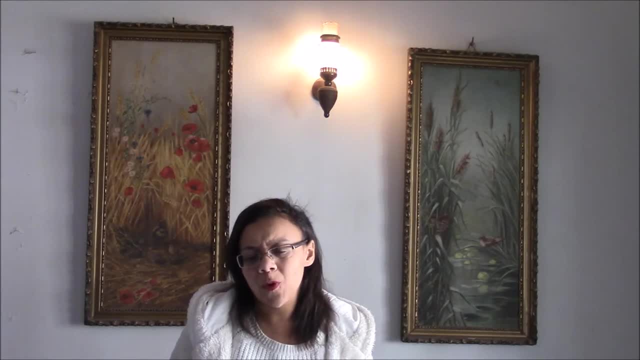 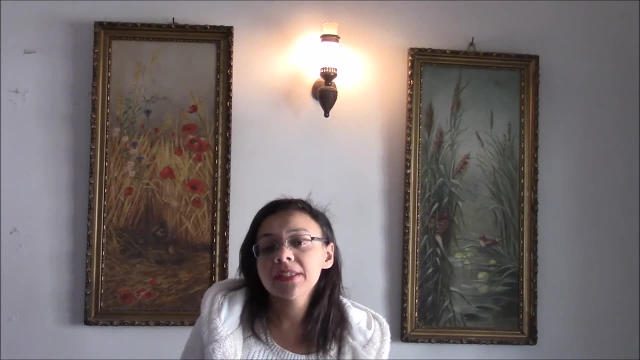 i hate the smell of vinegar. it makes me want to throw up. i hate the smell of vinegar. so, uh, yeah, that's how this works. so you only need to rinse um the shower head with the water, because it it's already soggy water, as we said in the um, the formula that we sew together, but and i'll have 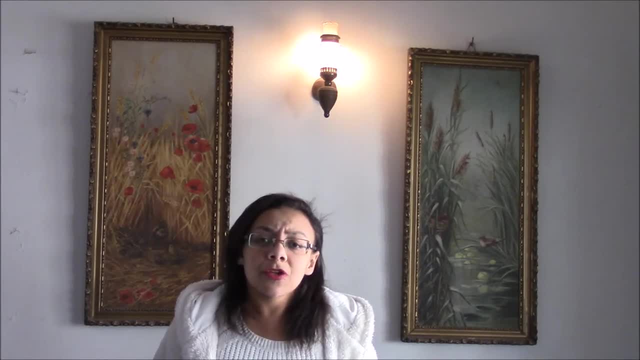 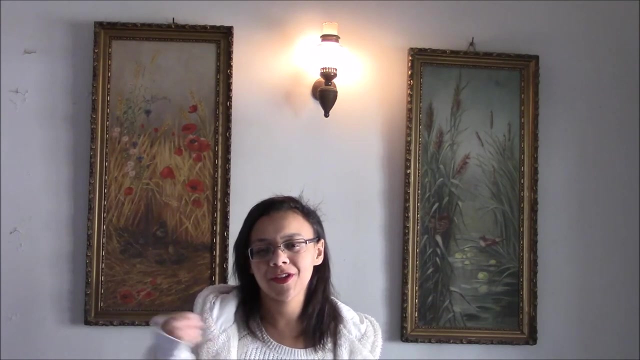 it on the screen too, just in case. so yeah, this is how it works, because the acids, any kind of acid admixture, will work with the calcium carbonate, that is, lime particles or calcium particles, that's participate, that's precipitated on the showerhead. so yeah, that's the all i have for today. 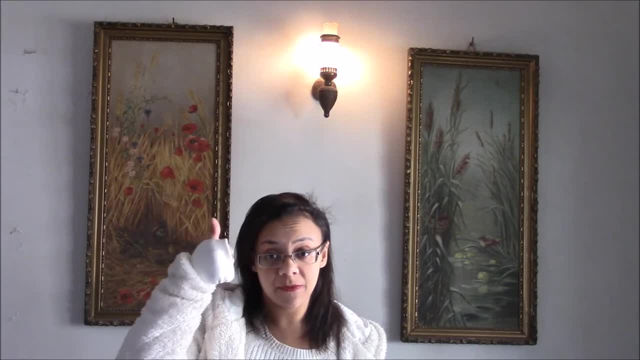 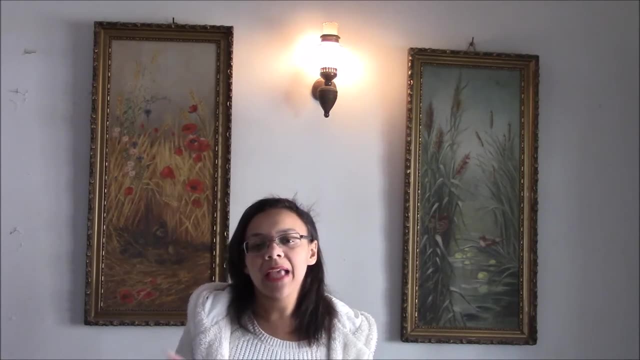 if you want to see a photo for this video, just give this video a big thumbs up so i can know that want to see a part two? and yeah, that's all for today. i try to be more active on this channel and actually i enjoy filming so much because so much was going on with me leaving my job that i 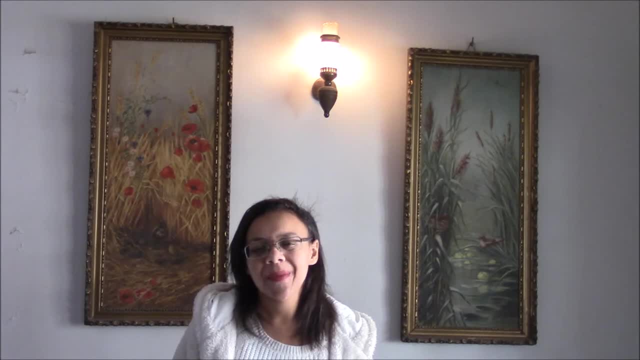 really loved. yeah, this is another talk for another time, but yeah, i love you guys so much and you make my day. um, i love- as crazy as it sounds- i love standing in front of a camera and talking to myself while everyone is outside and just, i like so much to talk to a camera like a crazy person. 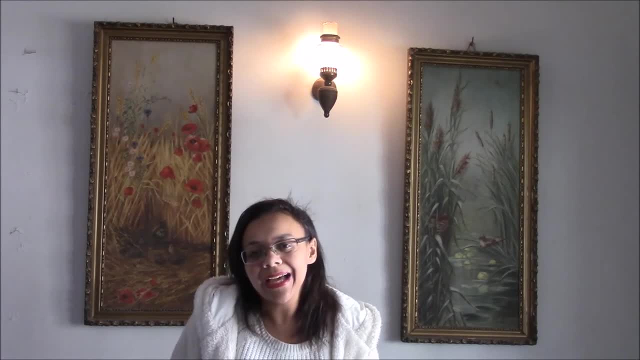 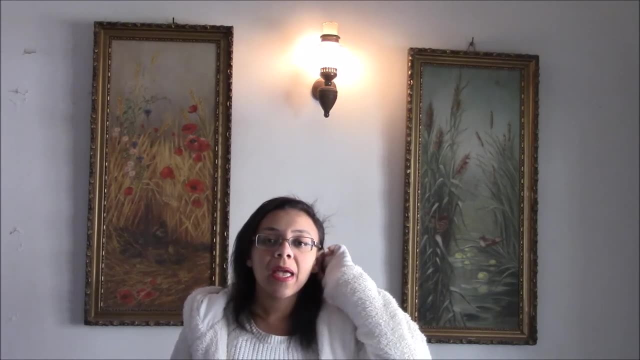 so i do what i like and yeah, so i'll try to be more active and thank you for subscribing and liking this video and comment down below which one you actually tried, if you tried any, or which one you want to try next. so thank you and that's all for today. 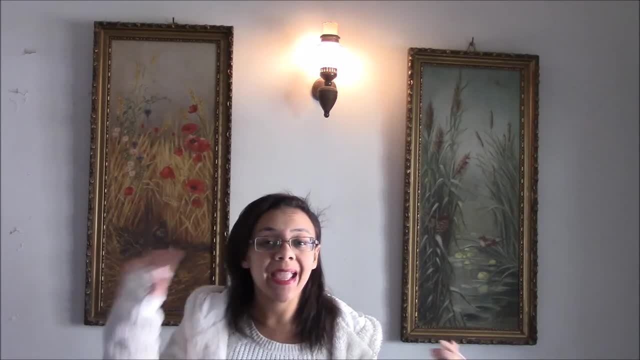 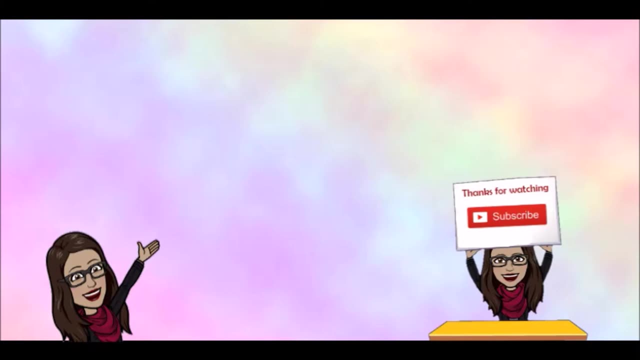 hope you enjoy it and hope you have a wonderful day, bye you.